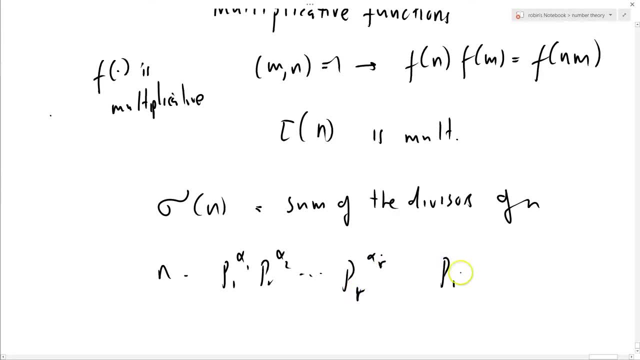 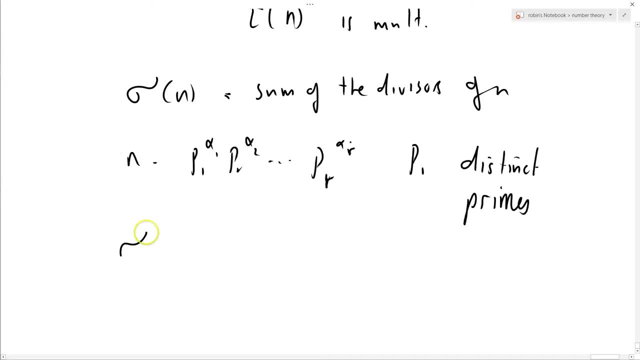 Actually we'll say pr to the alpha r, Where the pi are distinct primes. The formula we had was sigma of n equals. Let's see if I can get this right. It's p1 to the alpha 1 minus- Sorry, plus 1, minus 1, over p1 minus 1,. 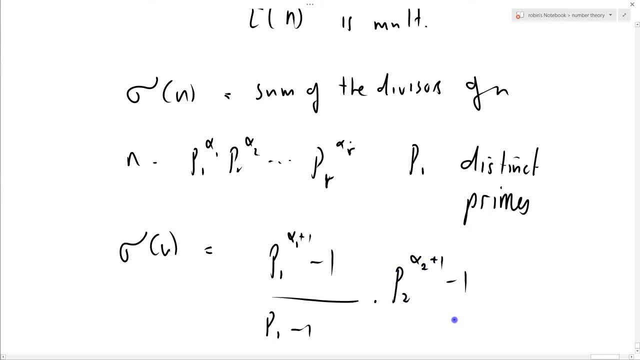 times p2 to the alpha 2, plus 1, minus 1, over p2.. times p2 to the alpha 2, plus 1, minus 1, over p2.. times p2 to the alpha 2, plus 1, minus 1, over p2.. 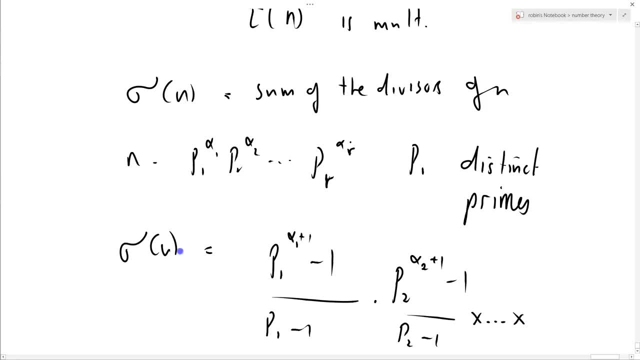 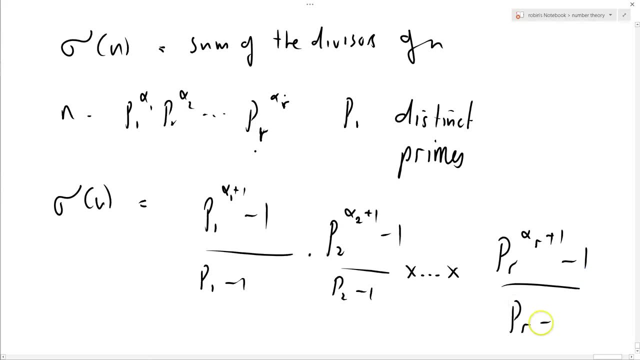 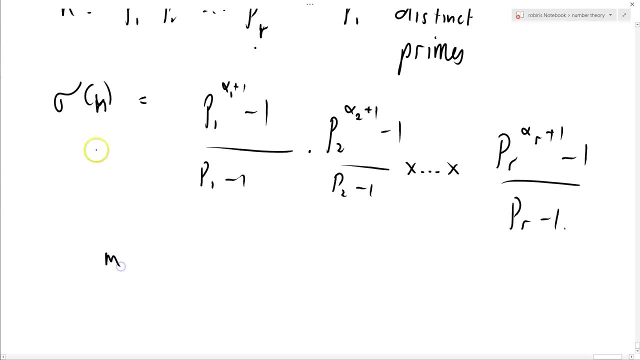 minus 1, times, all the way up to the final one, which is pr, to the alpha r. I keep on saying minus 1, plus 1, over pr minus 1.. And by the same logic as last time, if n equals that and m, so that's sigma of n. 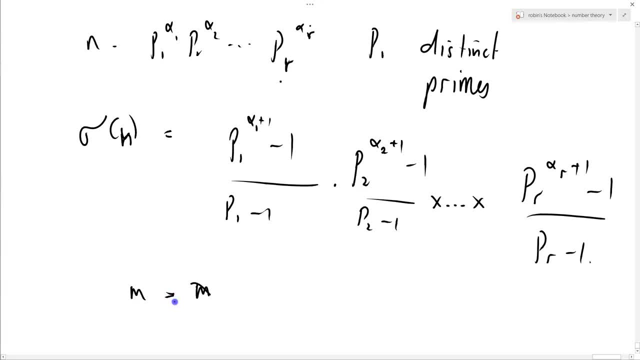 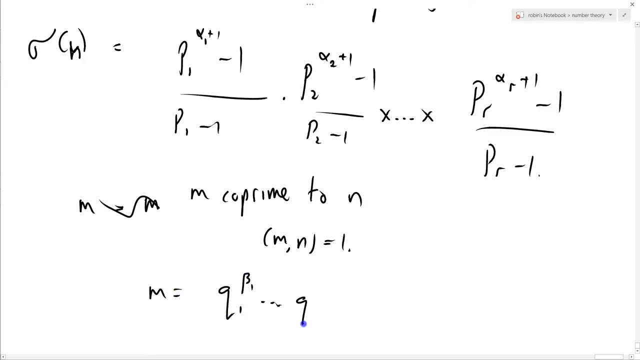 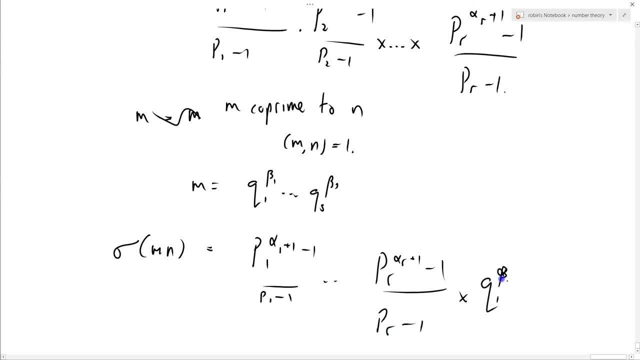 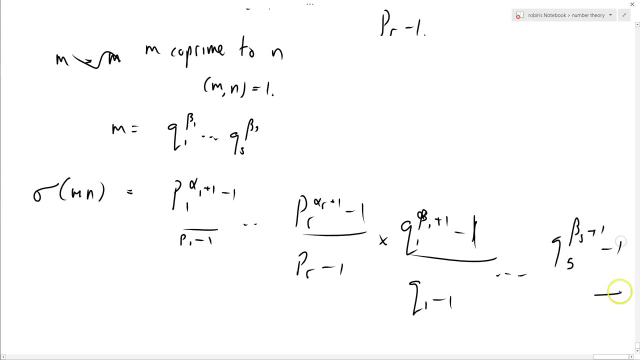 times. and now the q's q1. oh no, it's a beta q minus 1 over q1 minus 1 times all the way up to q. was it s beta? s plus 1 minus 1 over qs minus 1 equals sigma of m, sigma of n. so that checks out. 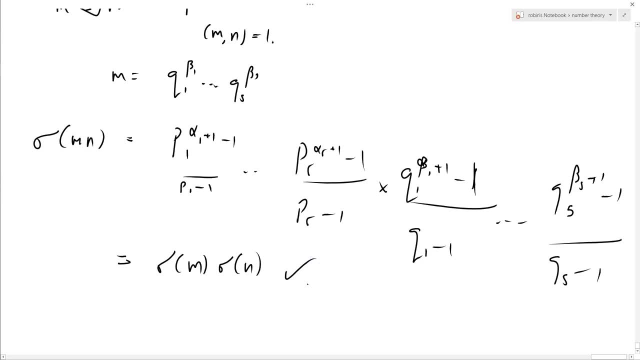 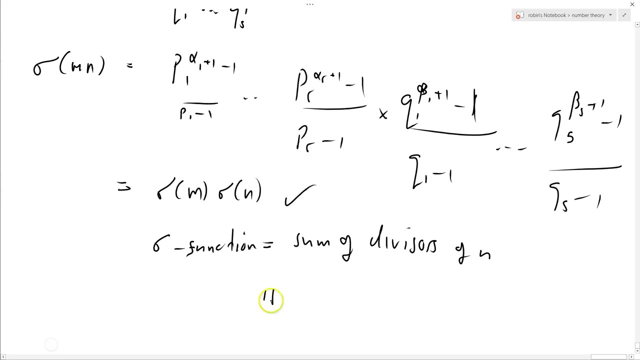 and sigma is now a multiplicative function. that's great. so the sigma function function equals sum of divisors of n is multiplicative, and that's why you do it like this. you do, you define the sigma function the way you do, so that the function itself is multiplicative. so, for example, if you're wondering, why do you include 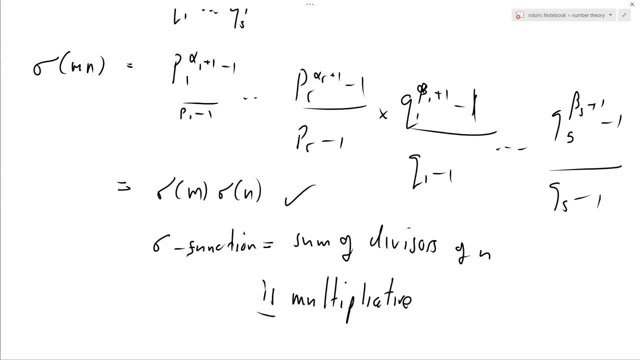 the number itself. why do you include n as a divisor of n when you're adding them all together? well, the answer is because the function that you get is multiplicative, and i'm going to stop there. 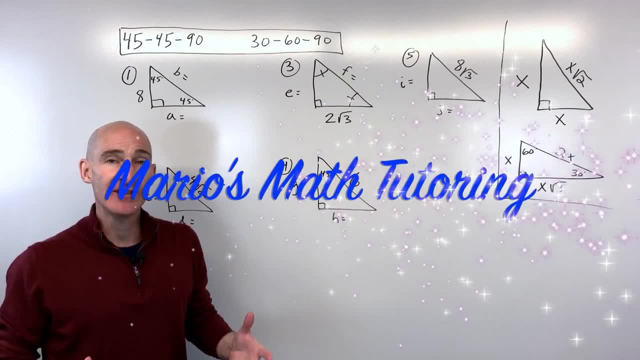 In this video we're going to talk about how to find the missing sides in the special right triangles: the 45-45-90 and the 30-60-90.. We're going to go through the 45-45-90 first. 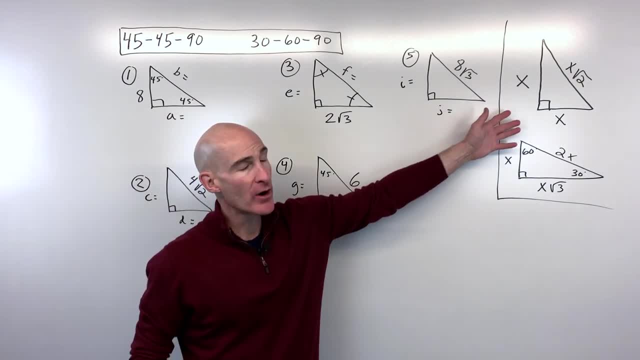 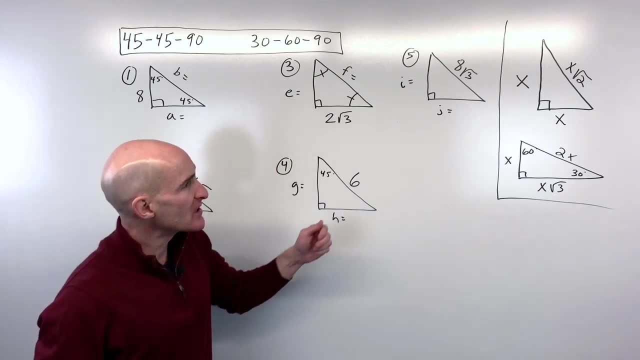 then we'll do the 30-60-90,. then I want to talk a little bit about where these side lengths come from. We can get into the theory a little bit if you're interested in that, and then we'll do some more problems at the end. So the first thing we want to talk about is the 45-45-90 triangle. So 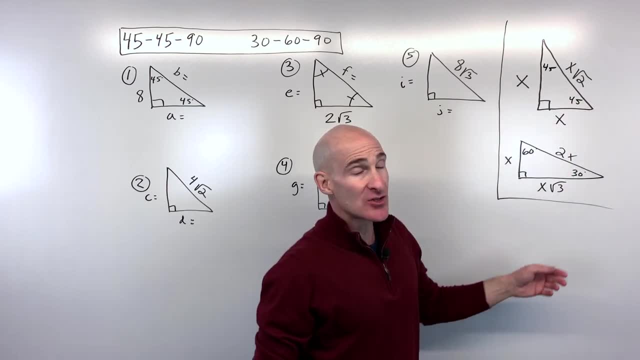 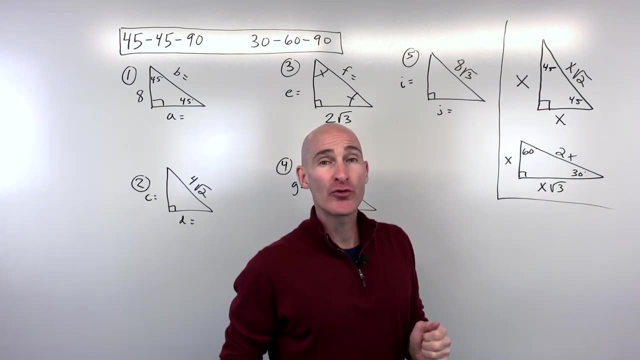 what you notice here is that it's an isosceles triangle. these base angles are congruent, and so that means that these two legs, or these two sides that make up that right angle, they're going to be congruent as well. So we refer to those sides as x and x. they're going to be the. 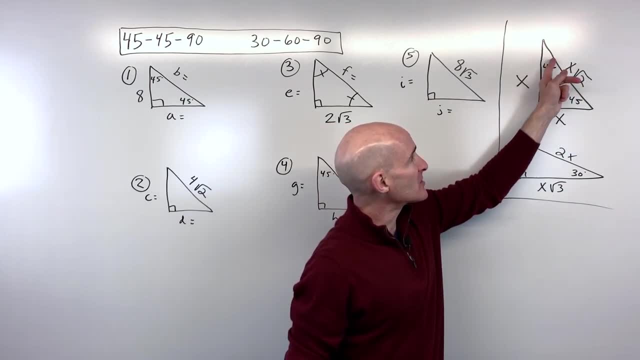 same. But to get to the hypotenuse, the side that's across from the right angle, you have to take that side or that leg and multiply by the square root of 2.. If you're going from the hypotenuse to the leg, you're going to want to divide by the square root of 2.. And just a quick. 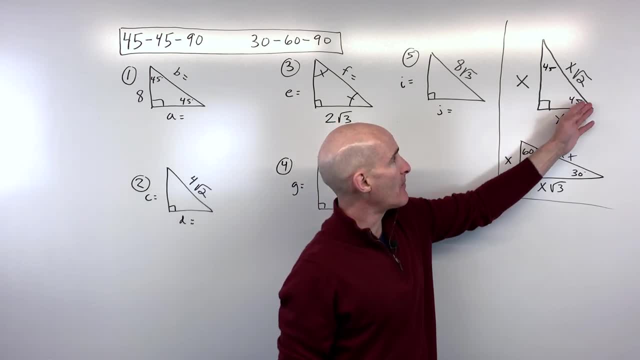 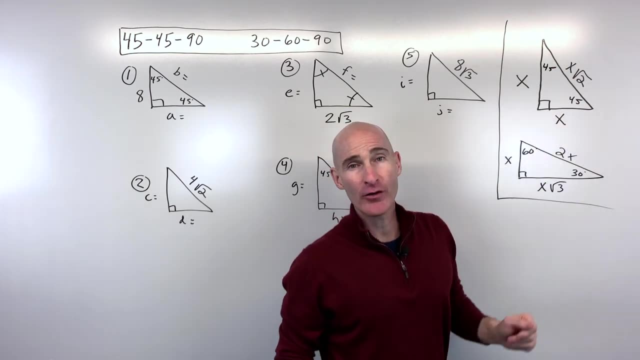 note square root of 2, it's about 1.2.. Which means that the hypotenuse is about 1.4 times longer than the leg. It's just that when we multiply by square root of 2, we're getting an exact value for that hypotenuse. So let's.